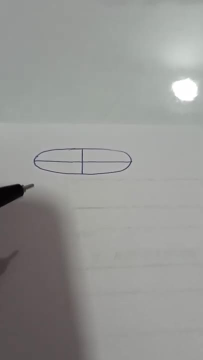 We have to find the equation of ellipse and we have given data and we have given data: the distance between the foci, so that the foci, the distance between the foci, is a eight unit, and distance between the directrix of jump- think tactics in happening- or directrix in happy or on. don't give each other distance. 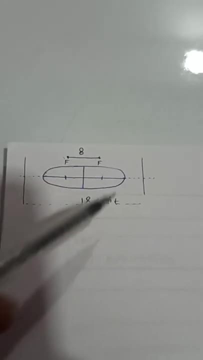 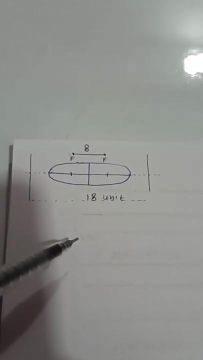 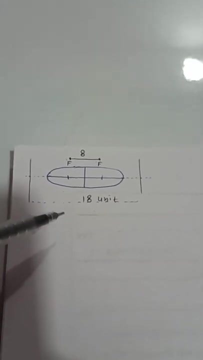 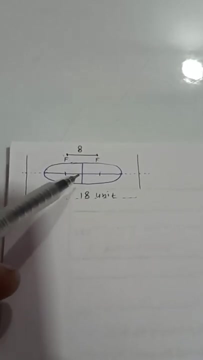 everywhere 18. so this is the rough geometry directrix distance: 18 unit and the foci distance is an 8 unit of. the correct way to solve this problem is to use a standard case and consider the center as 0,0 and you can take any other choice, either horizontal or vertical. 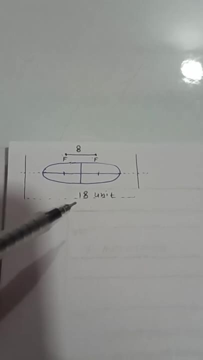 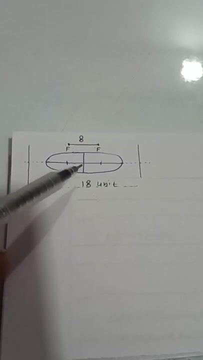 because you know that as you keep changing the center, you will get infinite equation of ellipses. but when such general cases are given, then you usually take the center as 0,0 and use any other case, either horizontal or vertical. so let's solve this question using horizontal method. 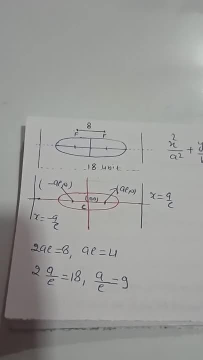 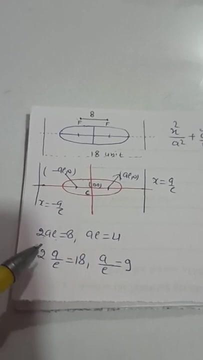 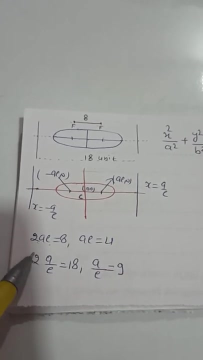 so in this way we have drawn a rough geometry. now distance is given as 8, so we will not take minus or plus. so we will get distance from A to E and total distance is 18. so if we take two times of directrix then its distance from center will be half. 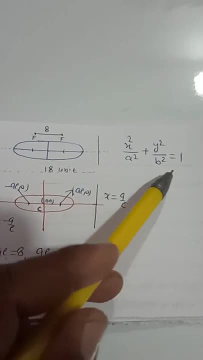 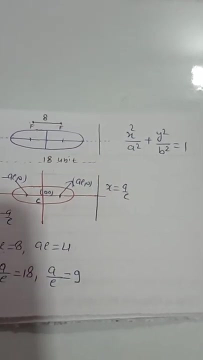 so we will get 9 and its equation is, as you can see here, this is its general equation. now what you have to do is you have to find the value of A and B and you have to find its equation. so here we have. A equals to 4. 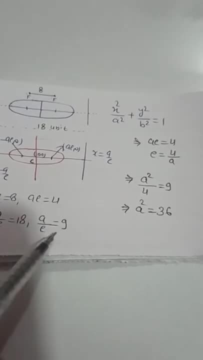 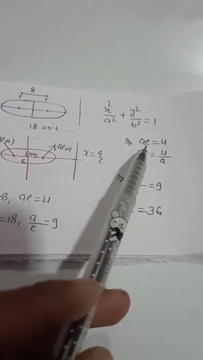 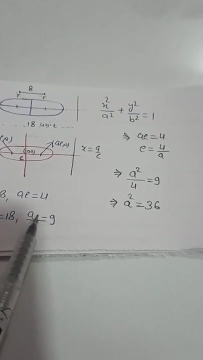 this is the first expression and from here you will see. so we will use this equation and leave E here. take A down, so keep E's value 4 upon A at this point, so A will go up. if you multiply then you will get A square, so the value of A square will be 36. 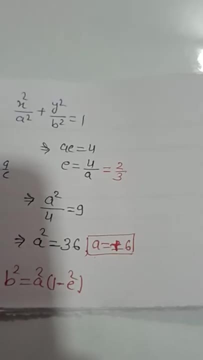 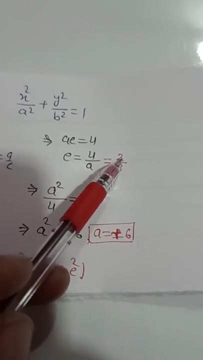 now what you have to find is you have to find B square. so from here you will get A equal to 6. take this 6 and keep it here, so E's centricity will be 2 by 3. now you have E and A. 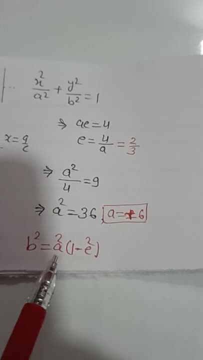 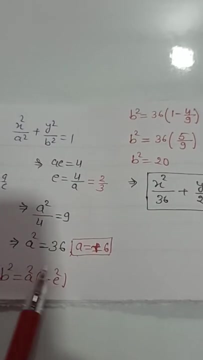 see this formula here: at the place of E, you will keep E's value. at the place of A, you will keep A. so from here we will find the value of B in this whole expression as you will substitute the values. so from here you will get, after LCM, 5 by 9. 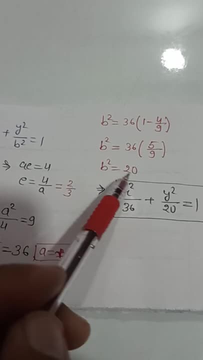 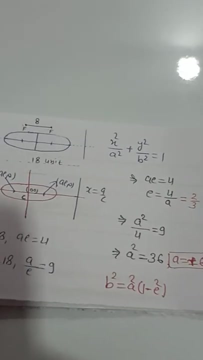 from 9, it will go 4 times. so B square, you will get 20. keep 36 at the place of A square and keep 20 at the place of B square. so in this way you will see the equation we have considered. we will get its equation in this form. and this is the equation of ellipse. 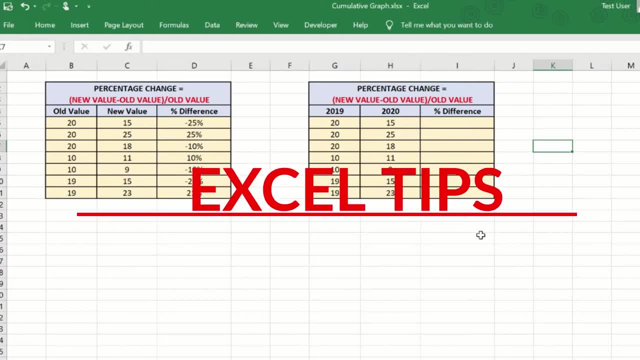 Hi everyone, and welcome to this video from Excel tips. In this video, you will see how to calculate the percentage change between two values using a very simple Excel formula. So in order to calculate percentage change, you will need two sets of data. One would be your old value and the other would be your new. 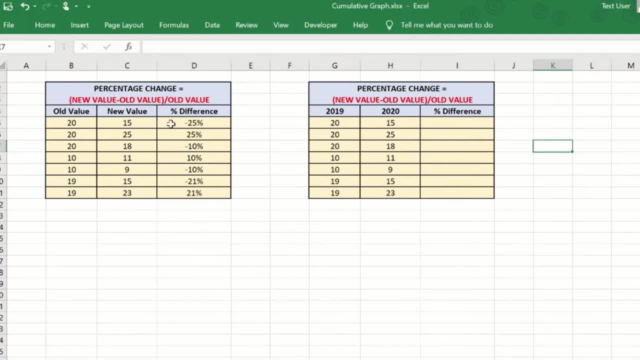 values and the results of the percentage difference can both either be positive or negative. If your new value is lesser than your old value, you would get a negative percentage difference, or which is also called as percentage decrease. In case your new value is greater than your old value, you would get a positive percentage difference. 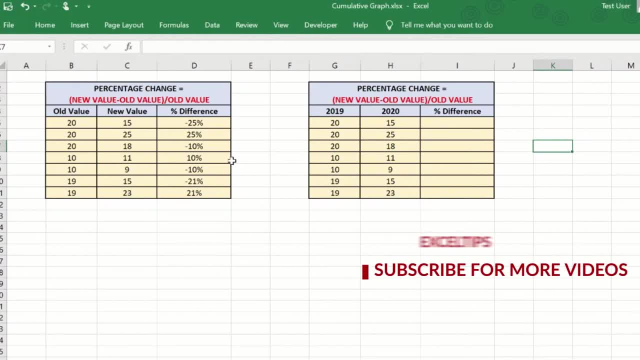 which is also known as percentage increase. So now that we know the different types of values or the different results, let's see how to calculate percentage change between two values using results that we can get from percentage difference. let us quickly look at the formula itself, as i